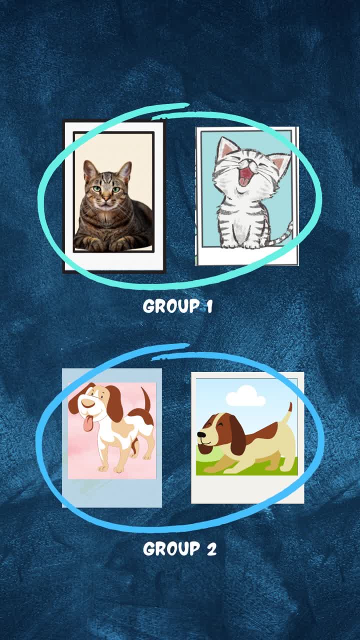 learning. we are not identifying whether it's a cat or dog, We are only grouping similar data together. 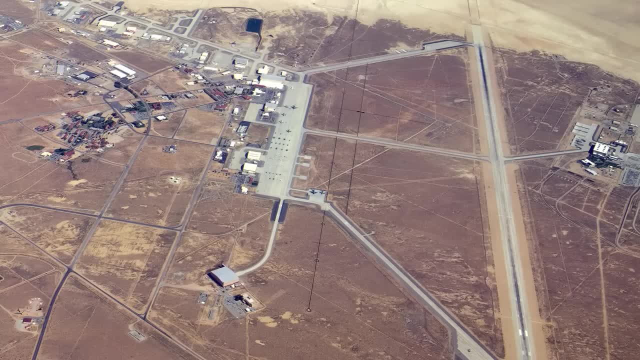 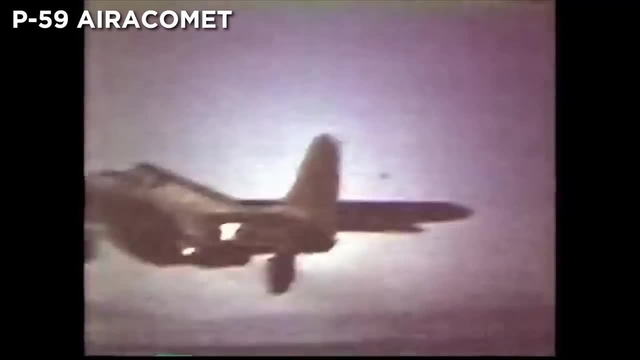 In 1942, the United States military was testing a top-secret plane at the Muroc Dry Lake bed in California, the current site of Edwards Air Force Base. The plane was called the P-59, and it was the first US jet engine plane. 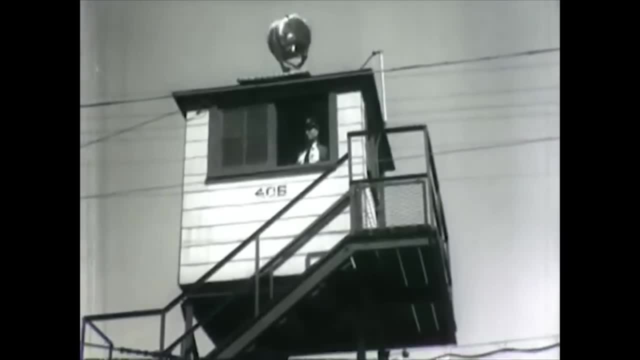 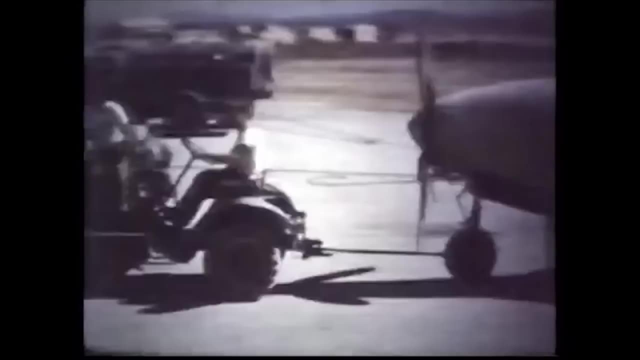 The secrecy around this thing was insane- almost the same level as the Manhattan Project. In fact, whenever they moved the plane around the base, they put a fake propeller on the front, because all planes before this were prop planes and a plane with no propeller would obviously get people's attention. 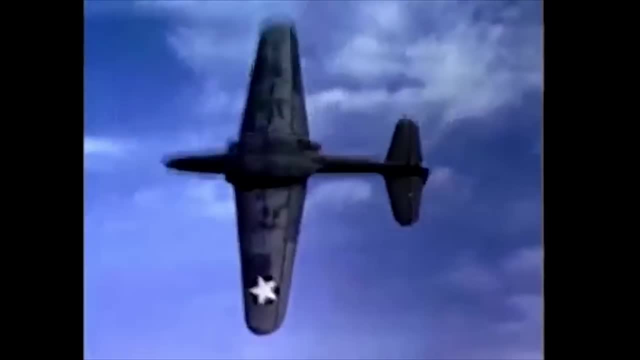 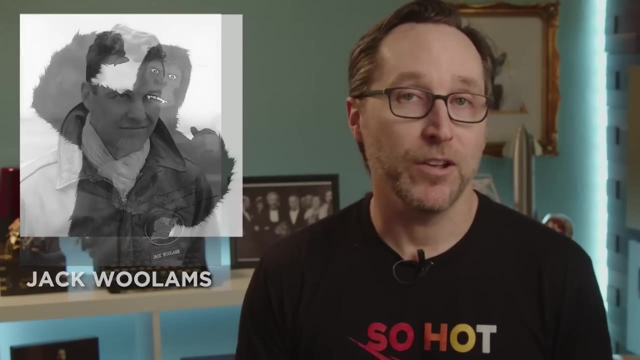 But of course they couldn't disguise it when it was in the air. so test pilot Jack Williams decided to take things to a bit more advanced level. What he did was he went to a costume shop in LA and he bought a gorilla suit, a derby hat and a big fake cigar. 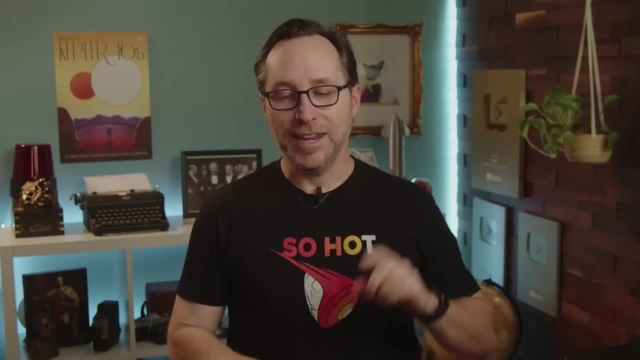 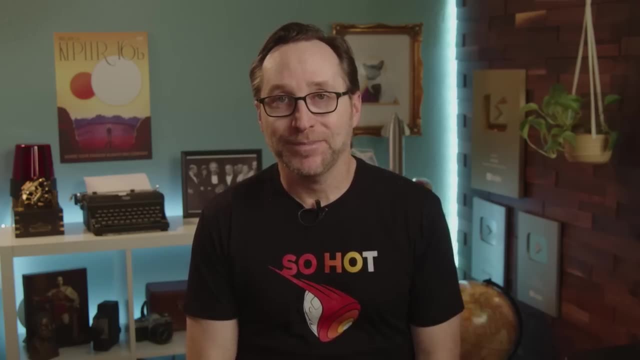 And he would wear this while he was out flying the plane. And he did this so that later on, when the other pilots told people what they saw, nobody would believe them. In fact, when they told people about it, they would get sent to the base psychologist and the base psychologists were in on it. 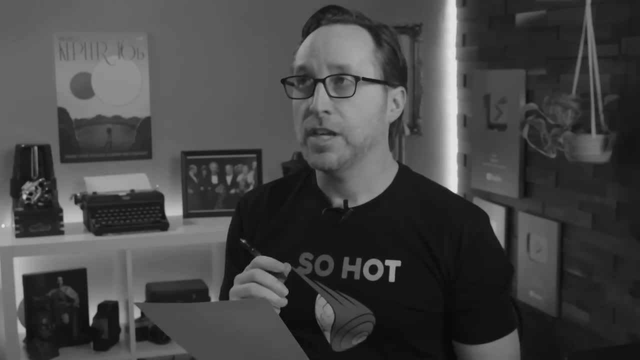 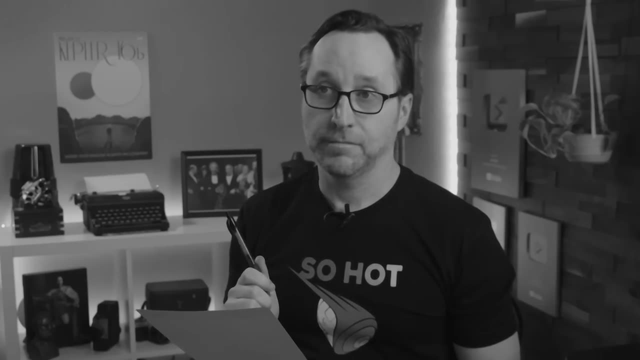 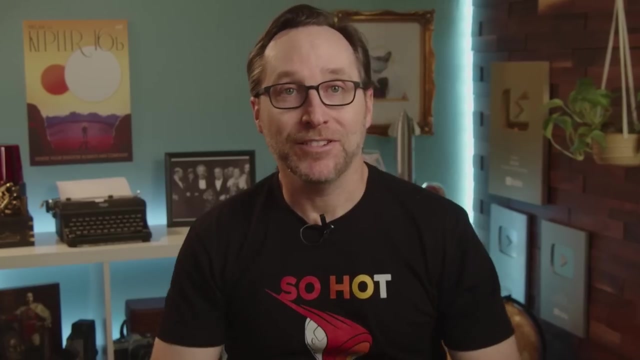 And they used it to convince them they were crazy. Okay, so you're telling me that you saw a plane with no propeller being flown by a gorilla wearing a hat? You can hear yourself right now. yes, They basically just gaslit an entire base full of pilots to convince them that they didn't see what they actually saw. 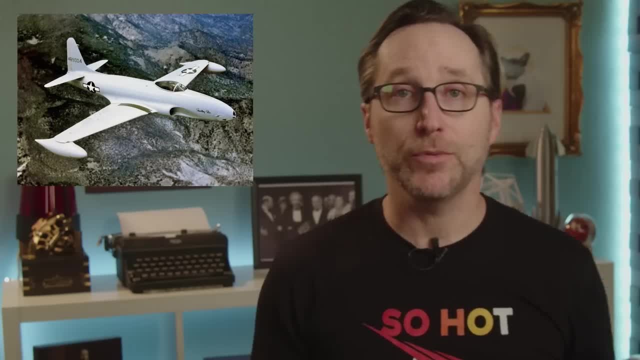 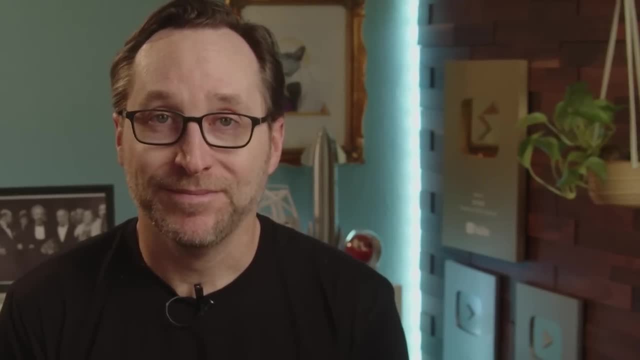 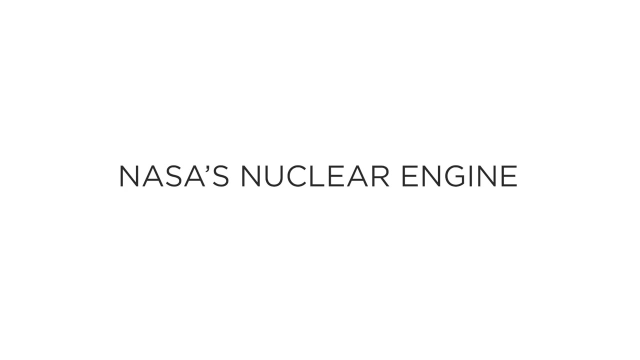 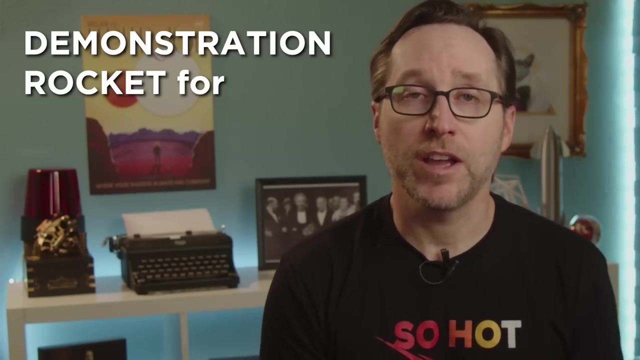 So we gotta talk about this. Back in January of this year, NASA, the National Aeronautics and Space Administration, announced they were teaming up with DARPA, the Defense Advanced Research Projects Agency, on a program called DRACO, which stands for Demonstration Rocket for Agile Cislunar Operations.